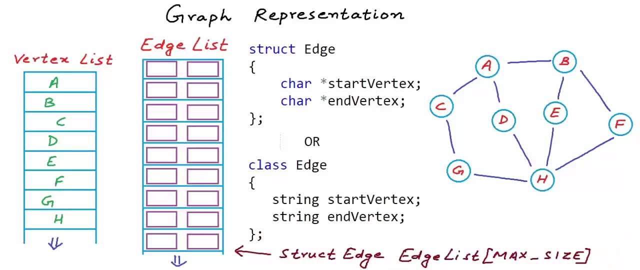 In these two definitions of edge that I have written here. in the first one I have used character pointers, because in C we typically use character pointers to store or refer to strings. We could use character array also In C++ or Java, where we can create classes. we have string available to us as a data type So we can use that also. So we can use any of these. for the fields We can use character pointer or character array. 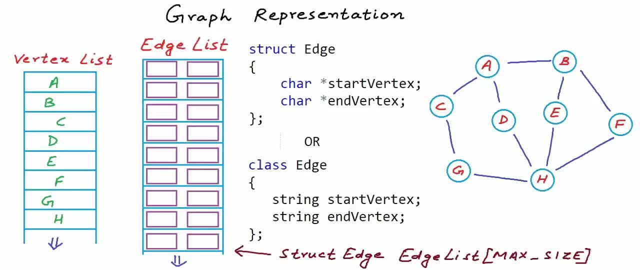 Or string data type, if it's available, Depends on how you want to design your implementation. Now let's fill this edge list here. for this example graph, Each row now here has two boxes. Let's say the first one is to store the start vertex and the second one is to store the end vertex. The graph that we have here is an undirected graph, So any vertex can be called start vertex and any vertex can be called end vertex. 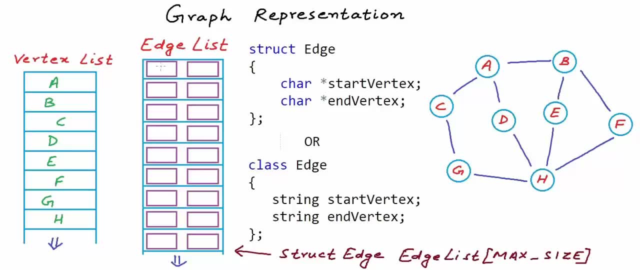 The order of the vertices is not important here. We have nine edges here: One between A and B, Another between A and C, Another between A and D, And then we have BE and BF. Instead of having BF as an entry, we could also have FB, But we just need one of them. And then we have CG, DH, EH and FH. 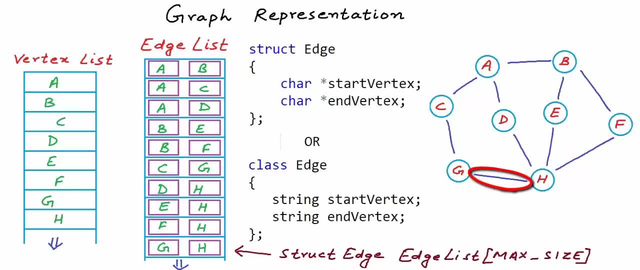 Actually there is one more. We also have GH. We have 10 edges in total here and not 9.. Now, once again, because this is an undirected graph, if we are saying that there is an edge from F to H, We are also saying that there is an edge from H to F. There is no need to have another entry as HF. We will unnecessarily be using extra memory. 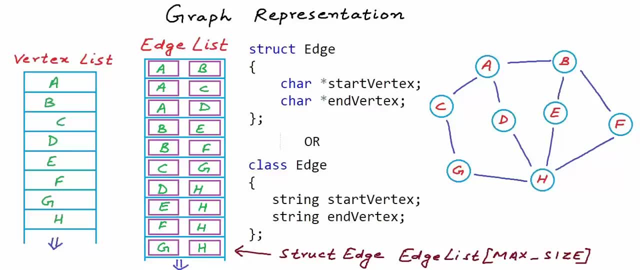 If this was a directed graph, FH and HF would have been the same, So we can use that as an extra memory. meant two different connections, which is the start vertex and which is the end vertex would have mattered. Maybe in case of undirected graphs, we should name the fields as first. 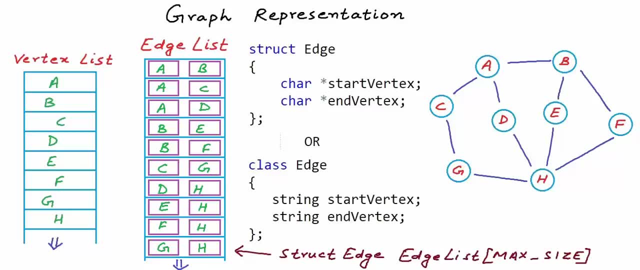 vertex and second vertex, and in case of directed graphs we should name the fields as start vertex and end vertex. Now our graph here could also be a weighted graph. We could have some cost or weight associated with the edges, As we know in an unweighted graph. cost of 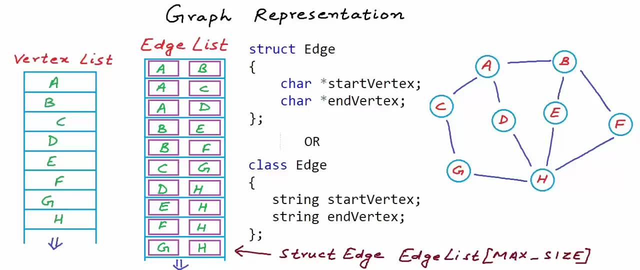 all the connections is equal, But in a weighted graph different connections would have different weight or different cost. Now, in this example graph here, I have associated some weights to these edges. Now how do you think we should store this data, the weight of edges? Well, 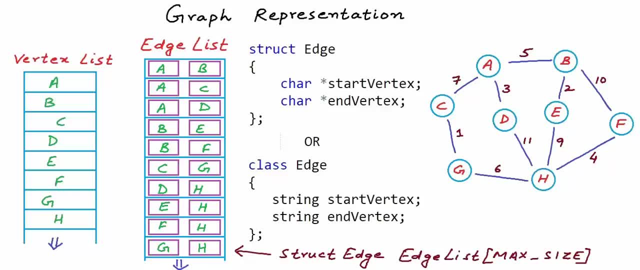 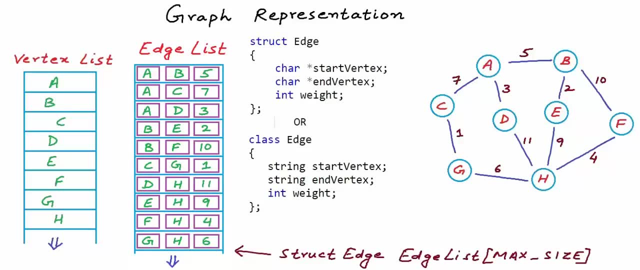 if the graph is weighted, we can have one more field in the edge object to store the weight. Now an entry in my edge list has three fields: one to store the start vertex, one to store the end vertex and one to store the start vertex. Now in this example graph we 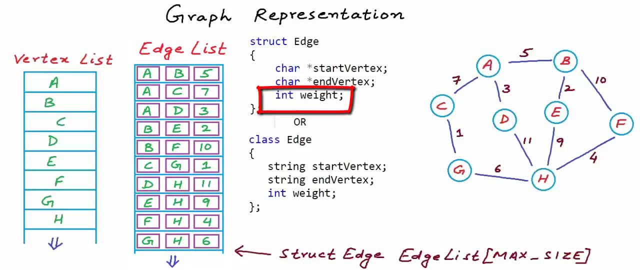 can have one more field to store the end vertex and one more to store the weight. So this is one possible way of storing a graph. We can simply create two lists, one to store the vertices and another to store the edges, But this is not very efficient For any possible. 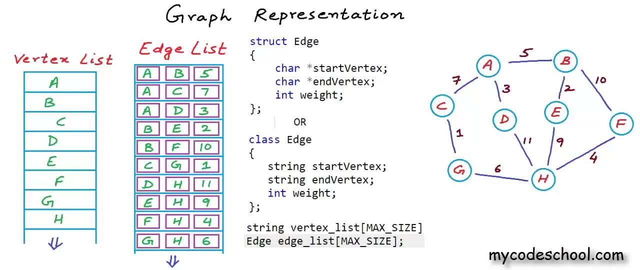 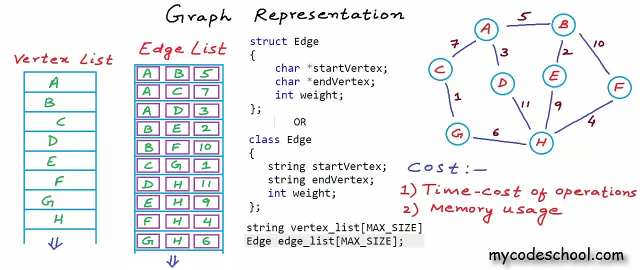 way of storing and organizing data. we must also see its cost, And when we say cost we mean two things: Time cost of various operations and time cost of various operations. So we collect the total amount of time and then Emmett uses it as a cost Time to collect the entire. 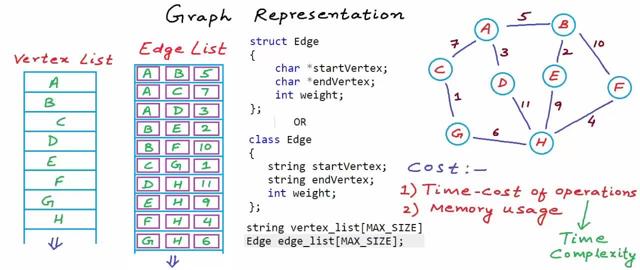 amount of time in theenviron, the entire object to store in one quick manner. So we estimate the total amount of time which was earned from all of these operations in one single way, one to size them, one to measure out. We measure the things that came out from every. 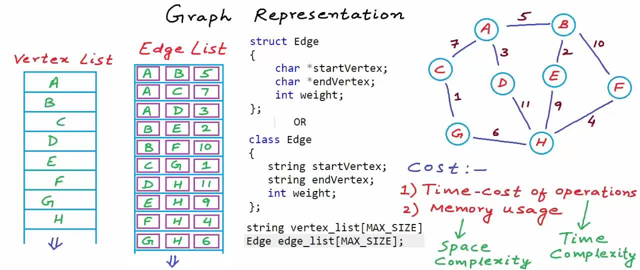 already know about Time and Space, Complexity Analysis and Big O Notation. If you want to revise some of these concepts, then you can check the description of this video for link to some lessons. We always want to minimize the time cost of most frequently performed operations and we always want to make sure that we do not consume unreasonably high memory. 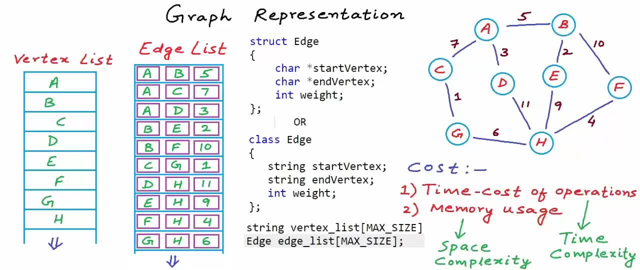 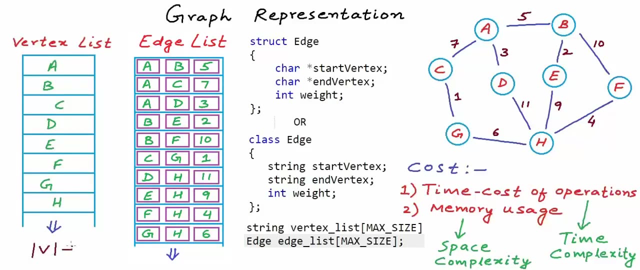 Okay, so let's now analyze this particular structure that we are trying to use to store our graph. Let's first discuss the memory usage For the first list, the vertex list. least number of rows needed or consumed would be equal to number of vertices. Now, each row. 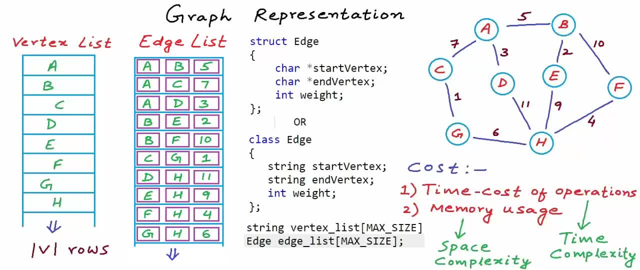 here in this vertex list is a name or string, and string can be of any length. Right now, all strings have just one character, because I simply named the nodes A, B, C and so on, But we could have names with multiple characters and because strings can be of different lengths. 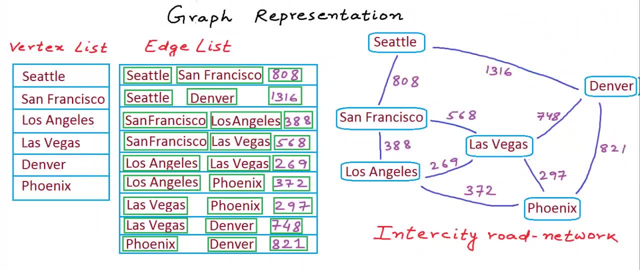 all rows may not be consuming the same amount of memory Like here. here I am showing an intra-city road network as a weighted graph. Cities are my nodes and road distances are my weights. Now for this graph. as you can see, names are of different lengths. 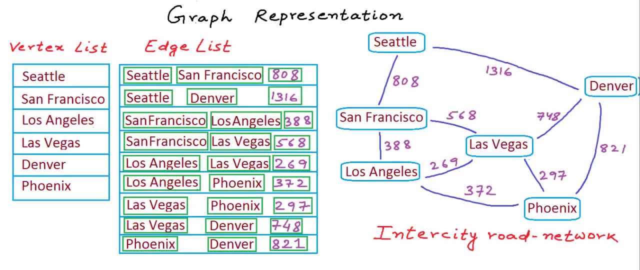 So all rows in vertex list or all rows in edge list would not cost us same. More characters will cost us more bytes, But we can safely assume that the names will not be too long. We can safely assume that in almost all practical scenarios average length of strings will. 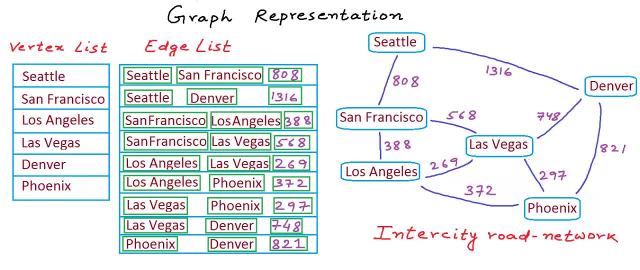 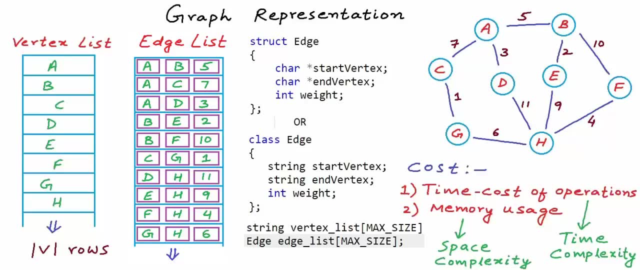 be a really small value. If we assume it to be always lesser than some constant, then the total space consumed in this vertex list will be proportional to the number of rows consumed, that is the number of vertices. Or in other words we can say that space complexity here is big O of number of vertices. 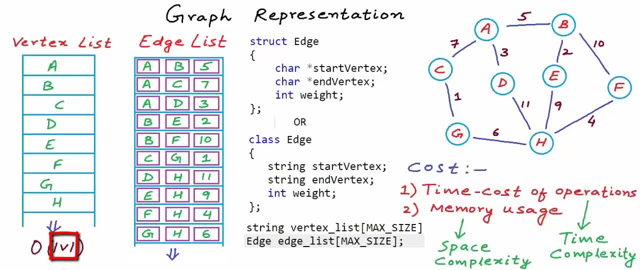 This is how we write number of vertices with two vertical bars. What we basically mean here is number of elements in set V. Now for the edge list. once again we are storing strings in first two fields of the edge object. So once again, each row here will not consume. 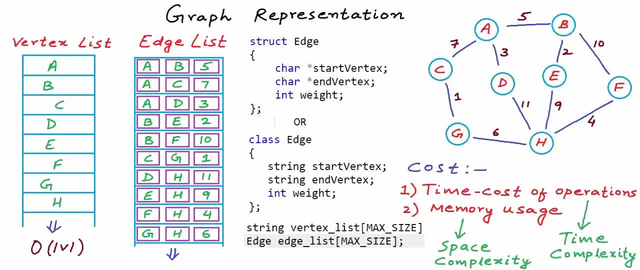 Same amount of memory. But if we are just storing the reference or pointer to a string, like here, in the first row, instead of having values filled in these two fields, we could have references or pointers to the names in the vertex list. If we will design things like this, each row will consume same memory. 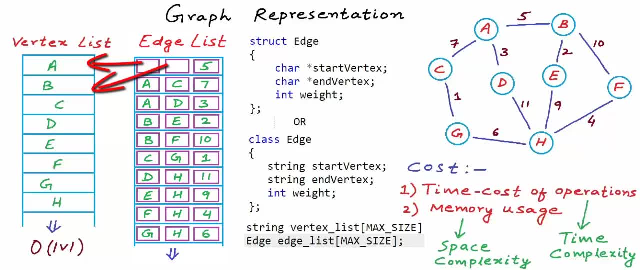 This, in fact, is better, because references in most cases would cost us a lot lesser than a copy of the name And as reference have the actual address of the string. and that's what we're doing when you're saying that start vertex and end vertex can be character pointers. 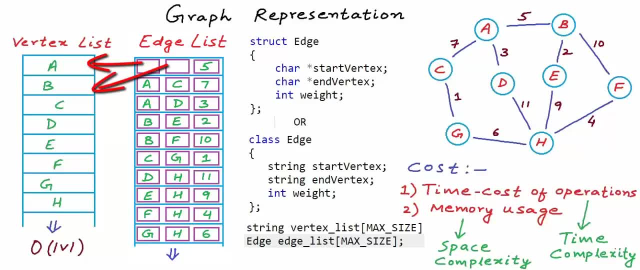 or maybe a better design would be simply having the index of the name or string in vertex list. Let's say A is at index 0 in the vertex list and B is at index 1 and C is at index 2, and I'll go on like this. Now, 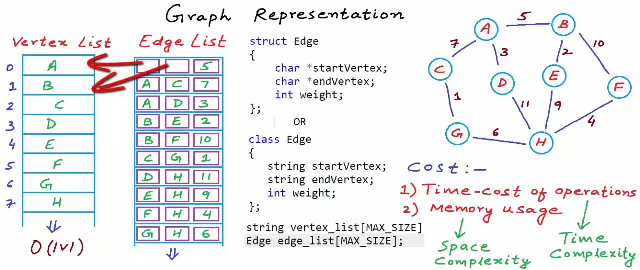 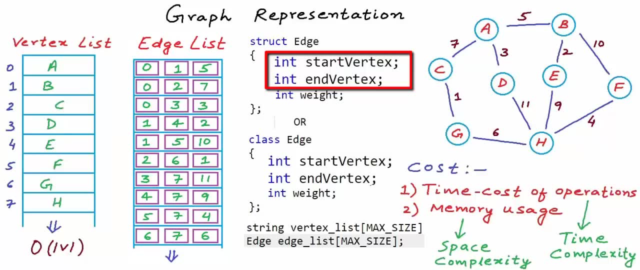 for start vertex and end vertex. we can have two integer fields. As you can see in both my definitions of edge, start vertex and end vertex are of type int now and in each row of edge list, first and second field are filled with integer values. I have filled in appropriate values of 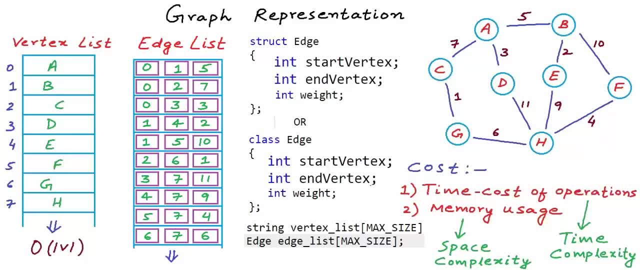 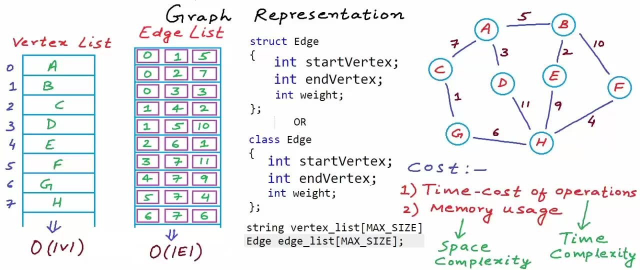 indices. This definitely is a better design and if you can see now, each row in edge list, edge list would cost us the same amount of memory. So overall space consumed in edge list would be proportional to number of edges, or in other words, space complexity. here is 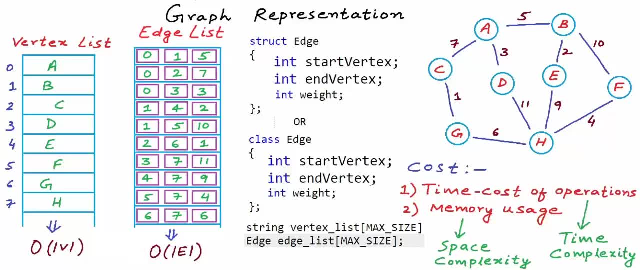 big O of number of edges. Okay, so this is analysis of our memory usage Overall. space complexity of this design would be big O of number of vertices plus number of edges. Is this memory usage unreasonably high? Well, we cannot do a lot better than this if we want to store a graph. 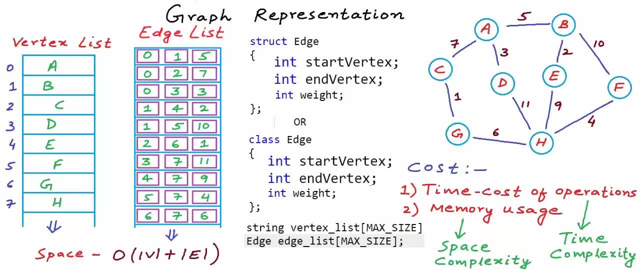 in computer's memory. So we are all right in terms of memory usage. Now let's discuss time, cost of operations. What do you think can be most frequently performed operations while working with graph? One of the most frequently performed operations while working with graph: 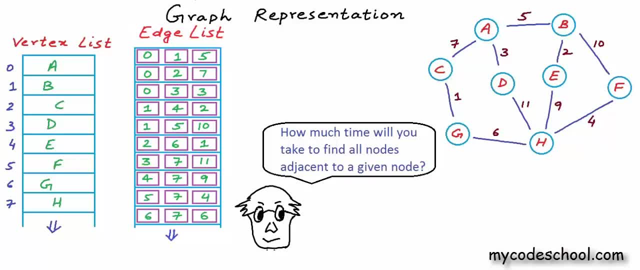 would be finding all nodes adjacent to a given node, That is, finding all nodes directly connected to a given node. What do you think would be time cost of finding all nodes directly connected to a given node? Well, we will have to scan the whole edge list. 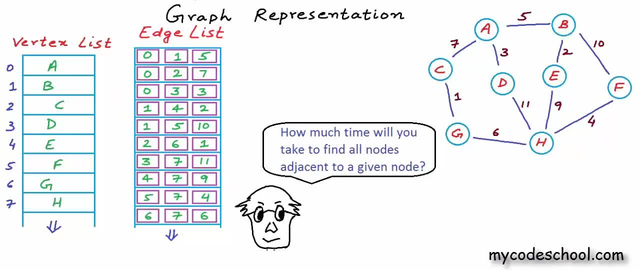 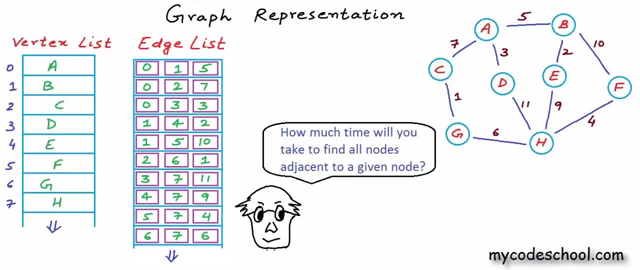 We will have to perform a linear search. We will have to go through all the entries in the list and see if the start or end node in the entry is our given node. For a directed graph, we would see if the start node in the entry is our given node or not. 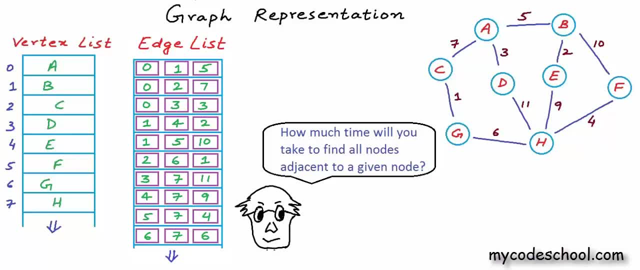 and for an undirected graph, we would see both the start as well as the end node. Running time would be proportional to number of edges, or in other words, time complexity of this operation would be big O of number of edges. Okay, now another frequently performed operation can be finding 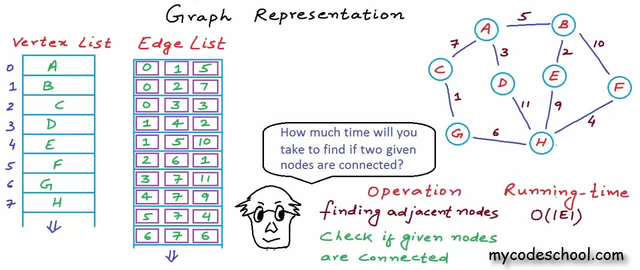 if two given nodes are connected or not. In this case also we will have to perform a linear search on the edge list. In worst case we will have to look at all the entries in the edge list. So worst case running time would be proportional to number of edges. So for this operation too, 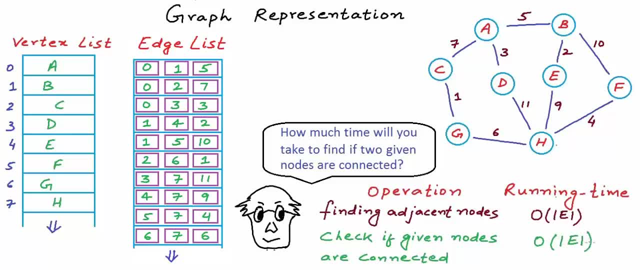 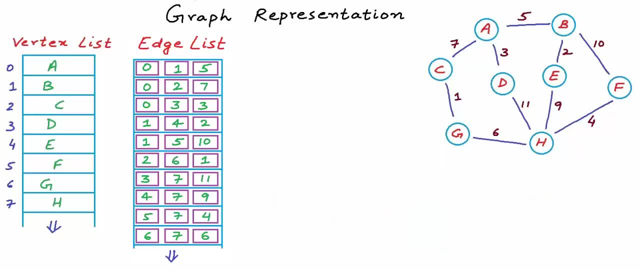 time. complexity is big O of number of edges. Now let's try to see how good or bad this running time big O of number of edges is, If you remember this discussion from our previous lesson, in a simple graph, in a graph with no self loop. 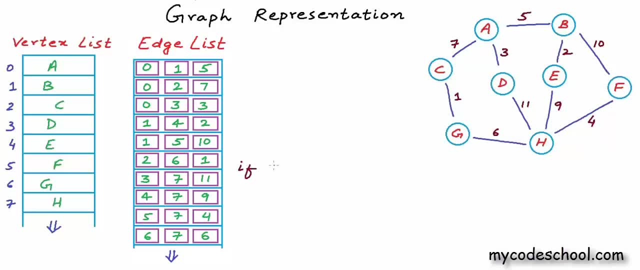 or multi edge. if number of vertices, that is the number of elements in set V, is equal to n, then maximum number of edges would be n into n minus 1. if the graph is directed, Each node will be connected to every other node and, of course, minimum number of edges can be 0.. 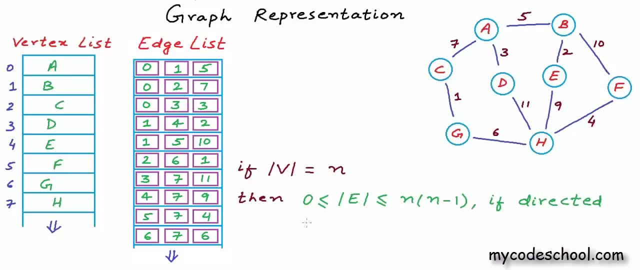 We can have a graph with no edge. Maximum number of edges would be n into n minus 1 by 2 if the graph is undirected. But all in all, if you can see, number of edges can go almost up to square of number of vertices. 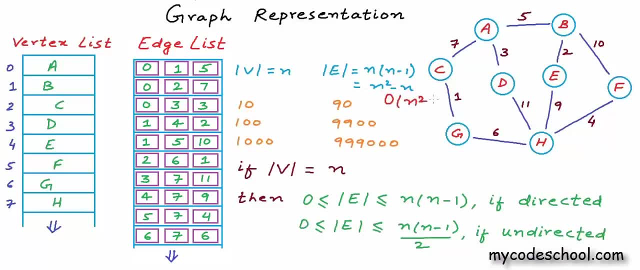 Number of edges can be of the order of square of number of vertices. Let's denote number of vertices here as small v, So number of edges can be of the order of v square In a graph. typically any operation running in order of number of.